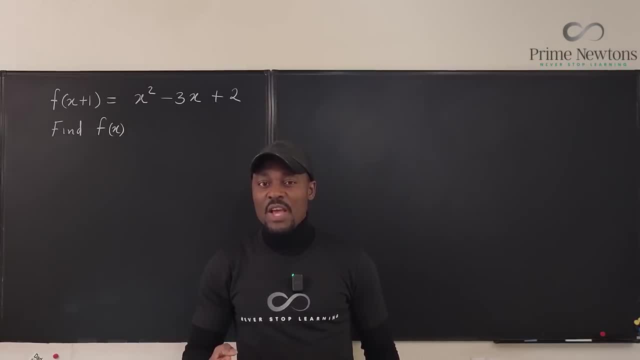 bill into it or quarters into it. What does it take When it takes that from you? what does it do to it? That's the meaning of a functional equation. What does F do to whatever you give to it? So, for example, if you give this machine X plus one, it will convert X plus one into this. 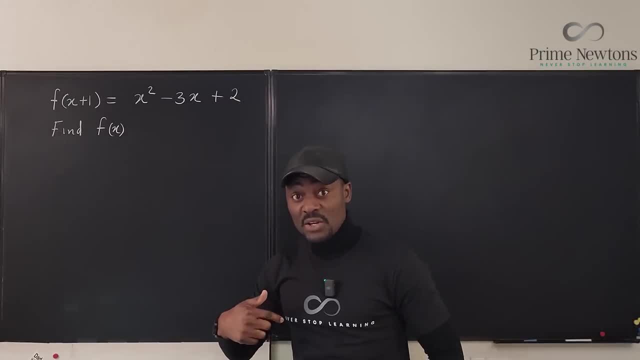 But you see, what it does to X plus one is not obvious. It's not obvious, It's not obvious. But we can make it obvious by doing this. Watch what I'm going to do, So I'm going to call this method one. 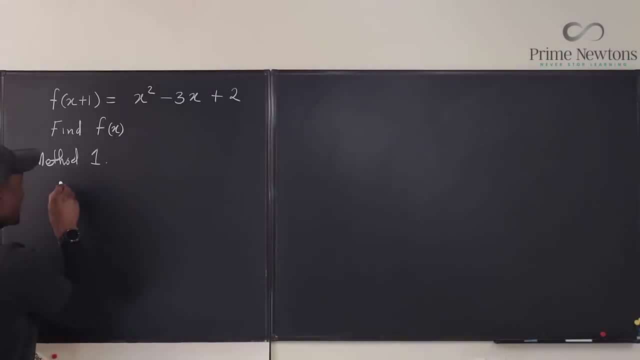 So what does it do to X plus one? See F of X plus one is equal to this, But I can write this in the factored form because this is a quadratic that I can factor to give me X minus one times X minus two. 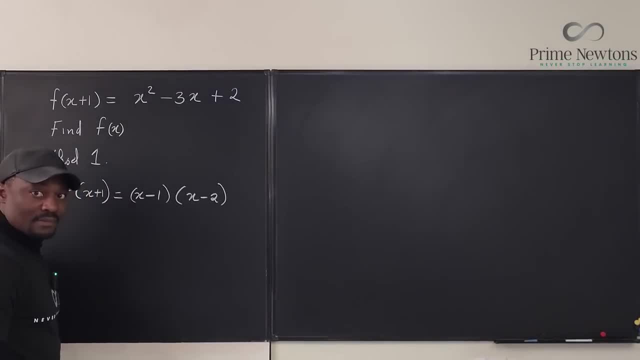 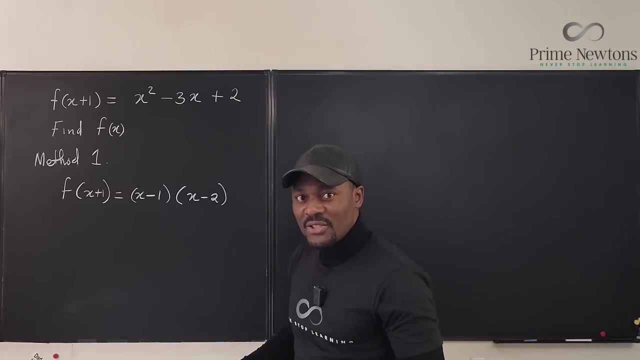 So that simply means whatever I give to this machine, it's still not obvious, because I cannot see this X plus one here. but I can create this X plus one here. How do I do it? It's just algebra. What would I do to X plus one to make it X minus one? Well, I can subtract two from here. So this: 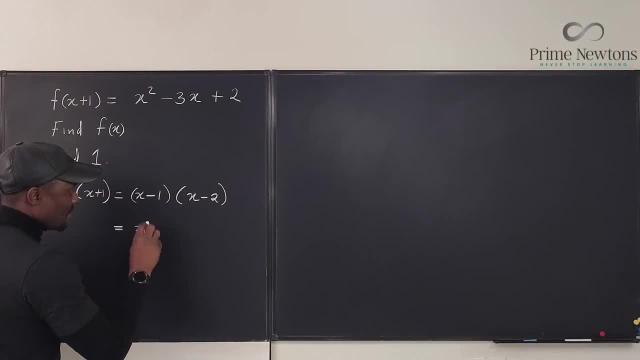 can be written as X plus one times X minus two. So that's the way to do it. So that's the way to do it as x plus one minus two. That's x minus one, And I'm multiplying it by x plus one. 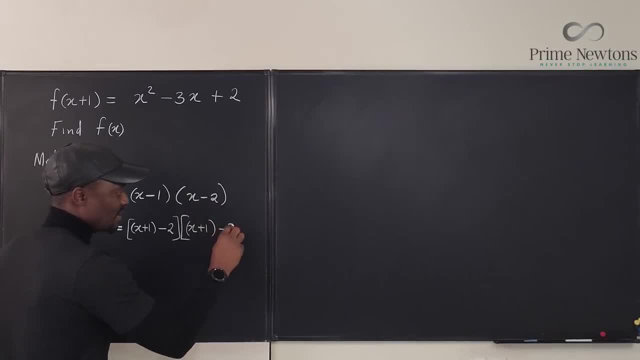 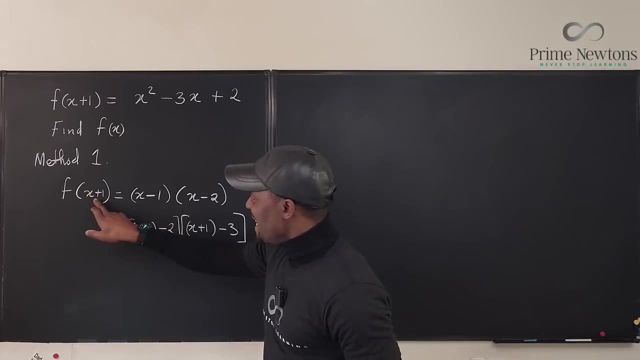 What would I do to x plus one? to make it x minus two, I subtract three from it. I have not changed what is on top here, But now it is obvious that what I gave the machine, this is what the machine did to it. 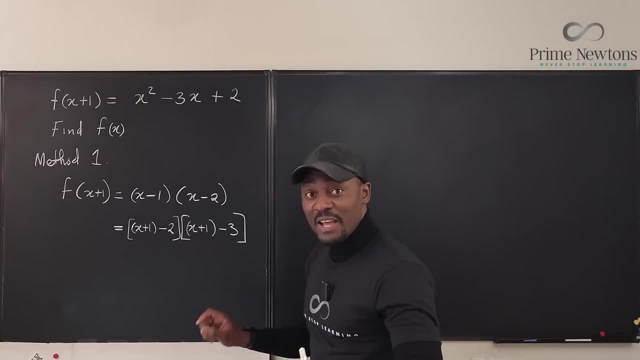 It took it, subtracted two from it and then multiplied it by the same thing, subtracting three from it. So I can boldly say: this is where you have to see the answer. That's why I call this the way of the masters. 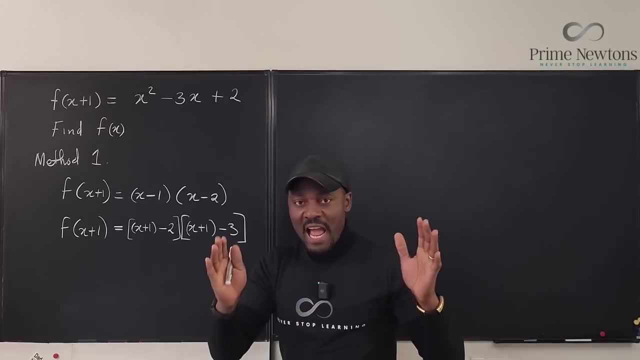 Whatever I give to the machine, it will put it as a product. One of it, it will take two away from it, And the other one, it will take three away from it. And that's how you get this. So I can say: 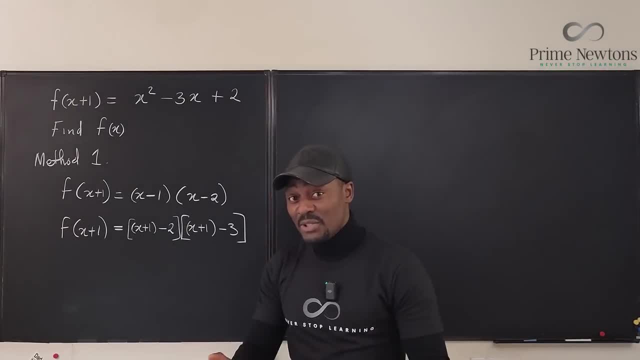 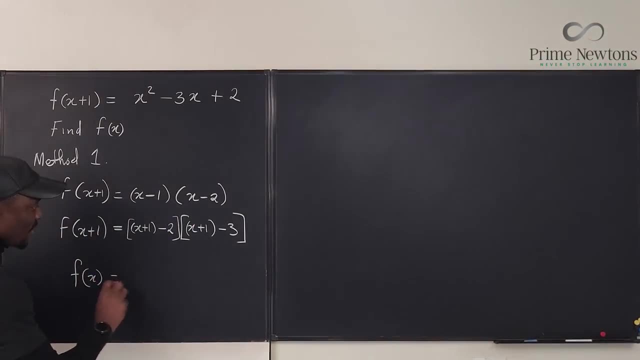 if I didn't give this machine x plus one? if I give the machine x, what would it do to x? The same thing, f of x will be x minus two times x minus three, which can show up in the form if I distribute this: 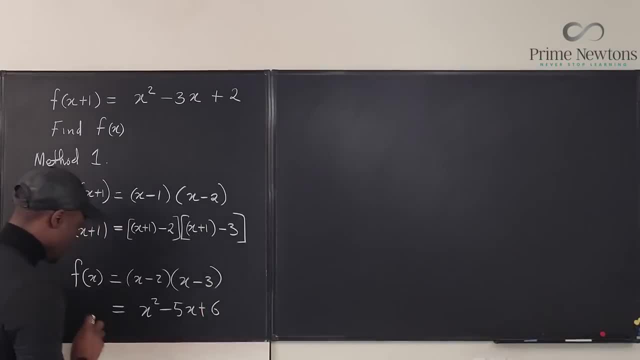 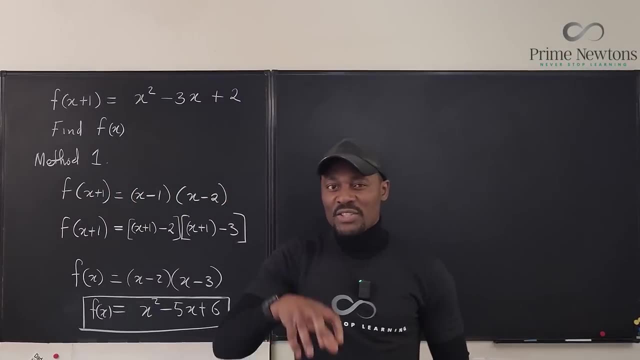 it is x squared minus five, x plus six, That's f of x. This is actually the answer to this problem. What does f do to its input? That is what you need to find. It has nothing to do with composition. What does f do to its input? 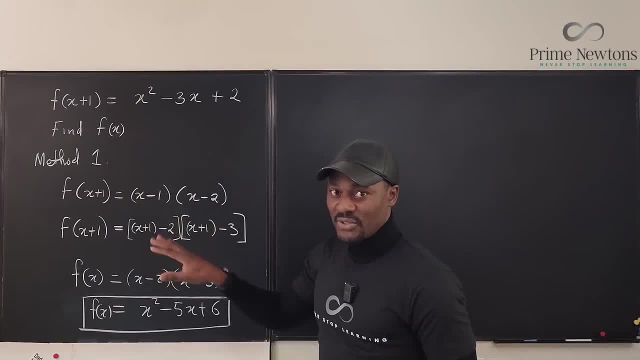 Okay, Now, this is the way of the masters, But the way I would recommend, which is applicable to every functional equation, that is this simple, because this is just substitution, we're not integrating and we're not doing some crazy stuff. But if it is just this, 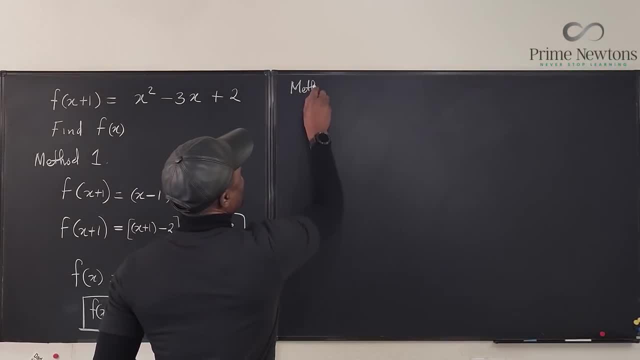 all you have to do is let's call this method two. We will need to do our t substitution. Okay, So we have. f of x plus one is equal to x squared minus three. x plus two. Now this doesn't look good. 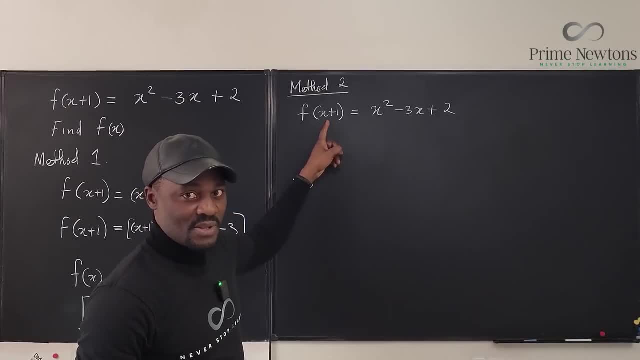 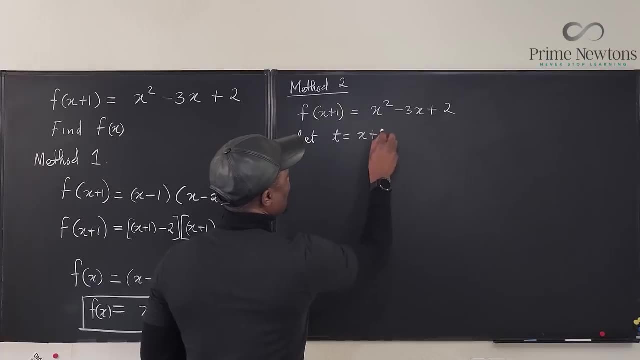 We want a single thing to be here, not a binomial. Okay, So let's say: let t be equal to x plus one, Then it means that x will be equal to t minus one If you move, subtract one from both sides. 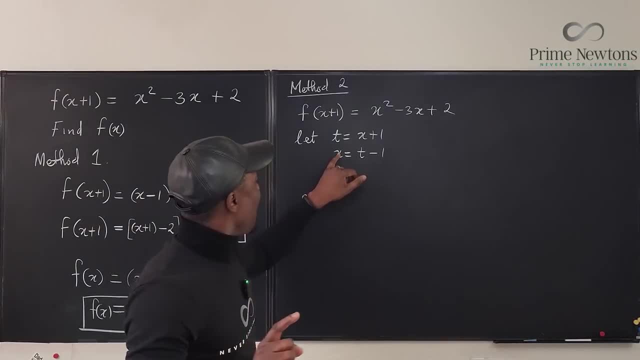 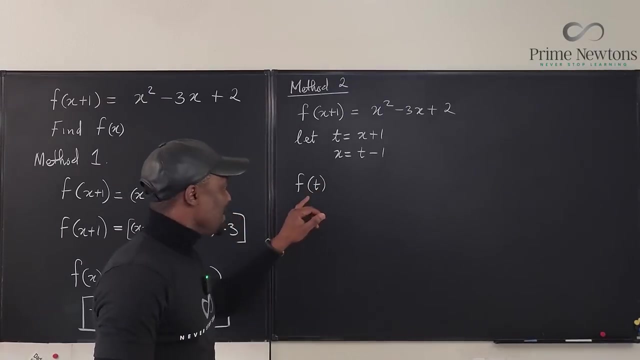 So anywhere I see x plus one, I'm going to put t, And anywhere I see x, I'm going to put t minus one. So let's go back here. It means f of t. Now look, The question we're asking is: t is now the input. 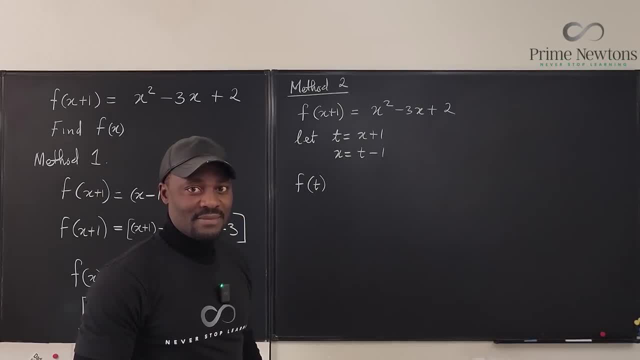 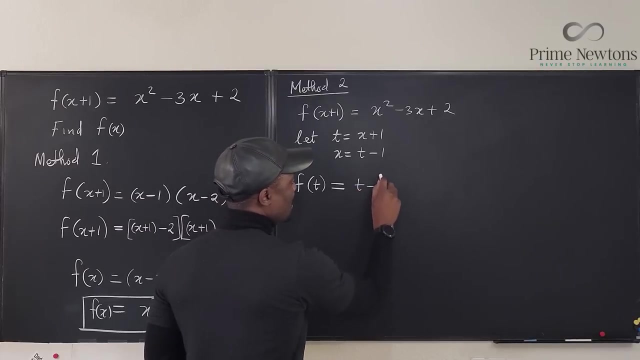 What would this machine do to t? That's all you're being asked. Do not overcomplicate this. And what does this mean? It means that this x squared will now be what is x now, T minus one? Everything now is in terms of t. 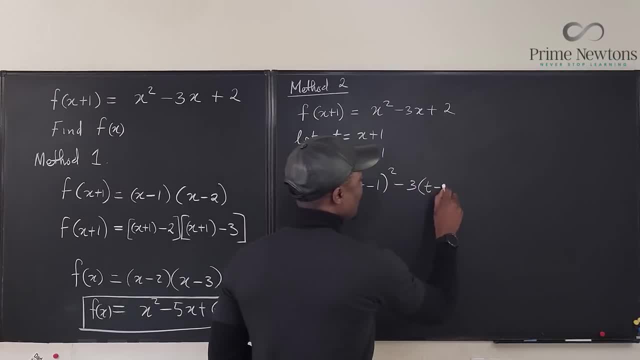 T minus one squared minus three times t minus one plus two. If we distribute this, it's going to be t squared minus two, t plus one, And if you distribute this, this is minus three t. This is plus three plus two. If you write this out. 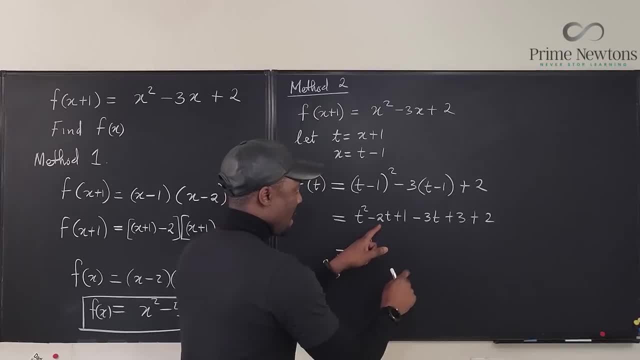 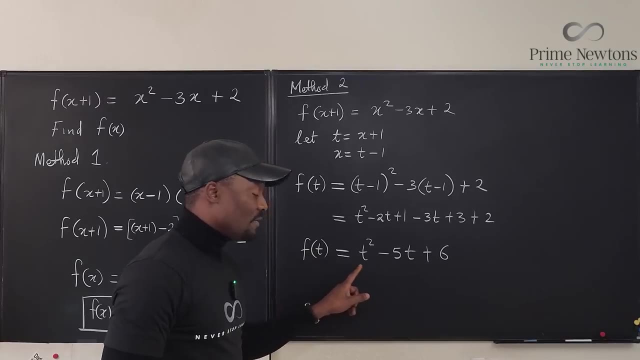 what does it mean? It means you have t squared minus two, t minus three, t is minus five t, And then one plus three plus two is plus six. So it means that whatever you give to f as an input, it will first square it. 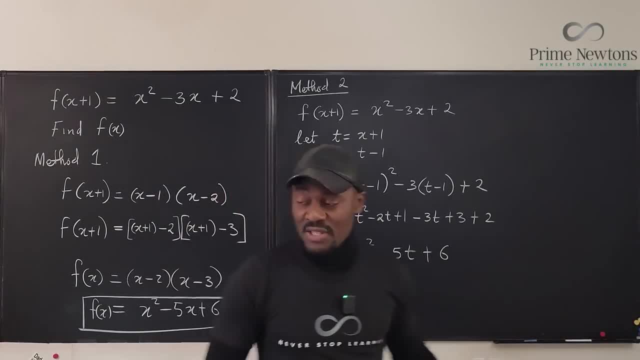 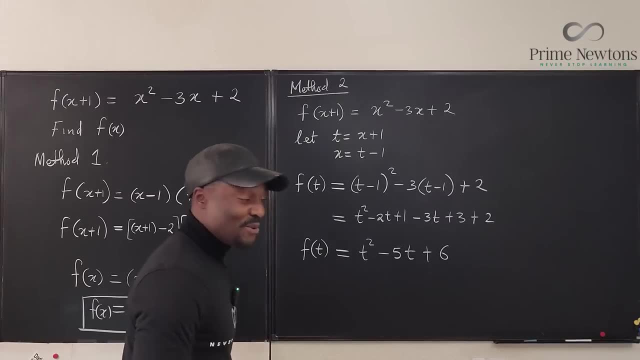 and then subtract five times of it and then add six to it. Does that look like this? It doesn't matter what letter you use as your substitution. Okay, the reason we use t is because we already used x here. We could have written this in terms of t. 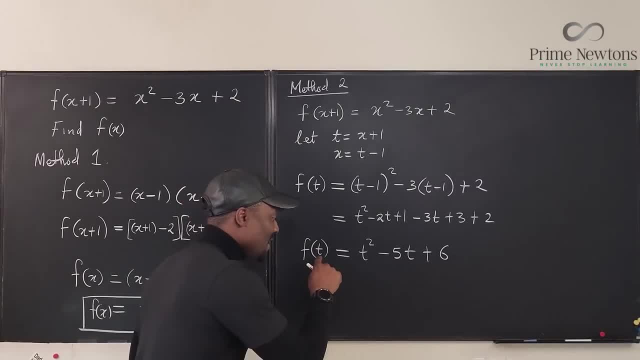 and then used x. eventually, It doesn't matter. Remember. what is here is the input. The independent variable could be any variable. Okay, therefore, f of x equals x squared minus five, x plus six. This is an input. This is an input. 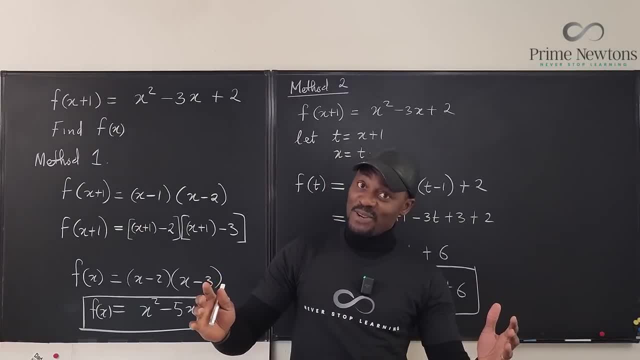 We could have used any letter. Okay, never stop learning. Those who stop learning stop living Bye-bye.